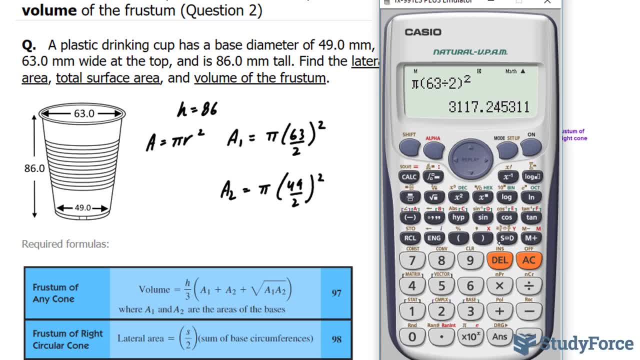 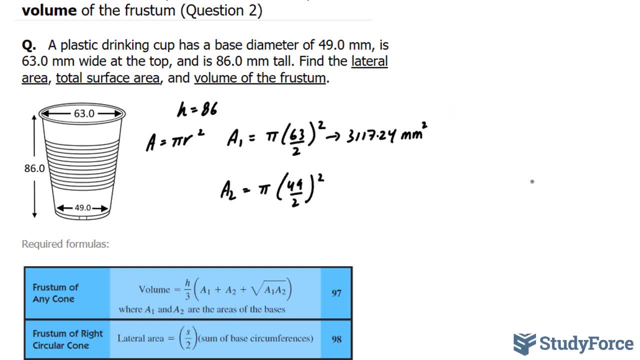 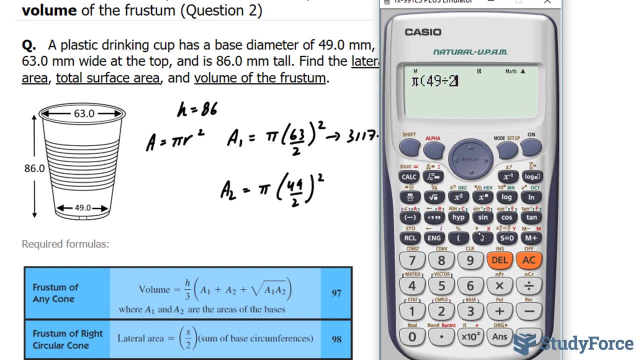 to the power of 2 is equal to approximately 3117.24 millimeters squared. Next, the area of the second base is pi bracket 49, divided by 2 to the power of 2, is equal to 1885.74.. 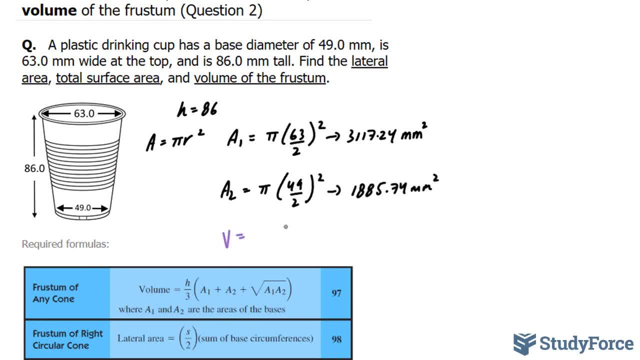 Using this formula, volume is equal to the height of 86, divided by 3.. a- 1 is 3117.24, plus 1885.74,, which is a square root of b squared. And the area of the second base is pi, bracket 49, divided by 2, to the power of 2,, which is 1.885.74.. using this formula, volume is equal to the height of 86, divided by 3.. a? 1 is 3117.24, plus 1.885.74,, whereas area 2 is 2 times the area of this shape. 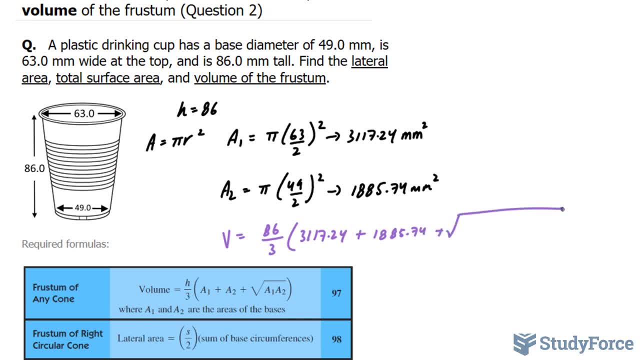 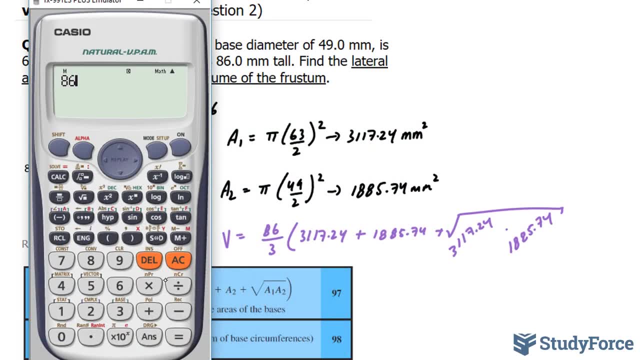 point seven, four plus the square root of the product of a1 and a2. using our calculator, eight, six divided by three, that covers this part times everything in the brackets: three, one, one, seven point two, four plus one, eight, eight, five point seven, four plus the square root of three, one, one, seven point two, four times. 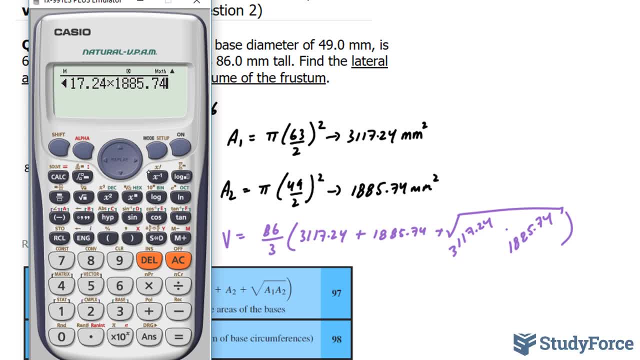 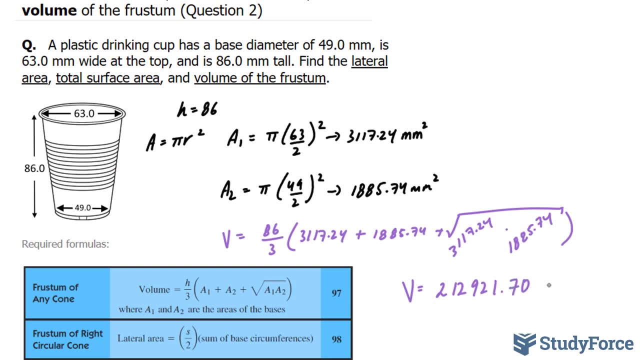 one, eight, eight, five, point seven, four. closing these brackets, we end up with a final volume of two hundred and twelve thousand nine hundred and twenty one, two hundred and twelve nine hundred and twenty one decimal seventy millimeters cubed. now that we found the volume, the next thing that we will find is the lateral area, so I'll 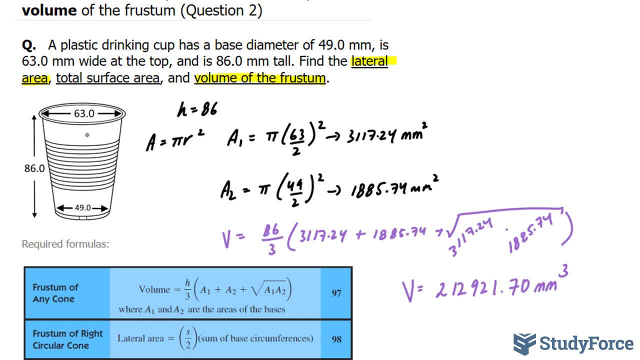 highlight what we've just found now. the lateral area refers to the surface area, except for the bases. so in our case we won't include this. neither will we include this. all we need to find is the area of the sleeve. we will use this formula to do that where lateral area is equal to s over 2 and s refers to the. 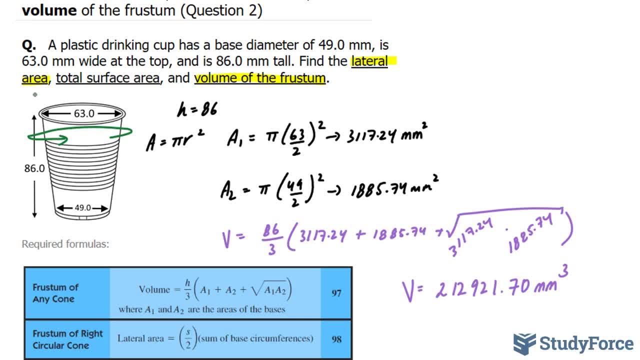 slant height. how do we find that? the way you find the slant height is? by the way you find the slant height is, by the way you find the slant height is to take a two-dimensional view of this three-dimensional shape, and if you look at this object in a 2d perspective, you'll actually create a. 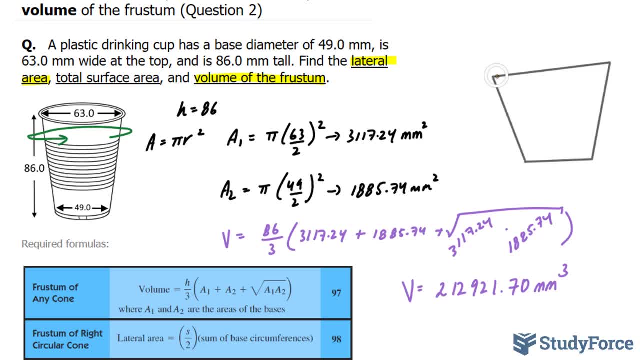 trapezoid. let me show you what I mean. where this represents 63, this represents 49. these two lines are parallel. obviously it's a trapezoid, even though it doesn't appear to be so. it's a crude drawing, and the height will be 86 to. 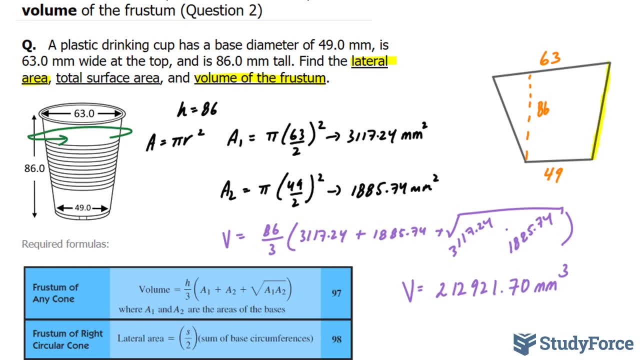 find the slant height, which will be highlighted in yellow, you'll need to use the Pythagorean theorem. take a look. this is also a right triangle, as is this one. we know that this is 86, but we don't know this. to find out the length from here to here, what we have to do is take. 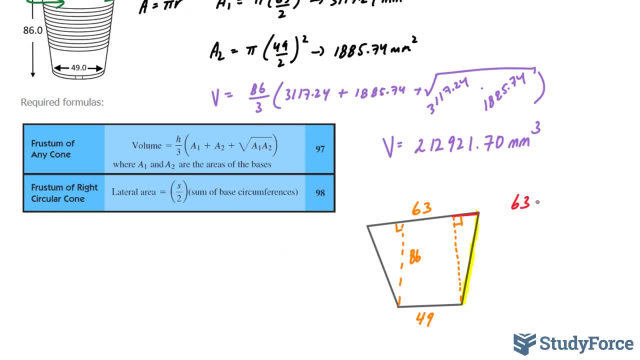 63, the total length from here to here. subtract it from 49 and that will leave us with two equal parts. so 63 minus 49 is equal to 14, and to find these- they're both equal- we divide by 2 and it gives us 7, so this is 7 and this is 7. 7 plus 49 plus 7 gives us 63. 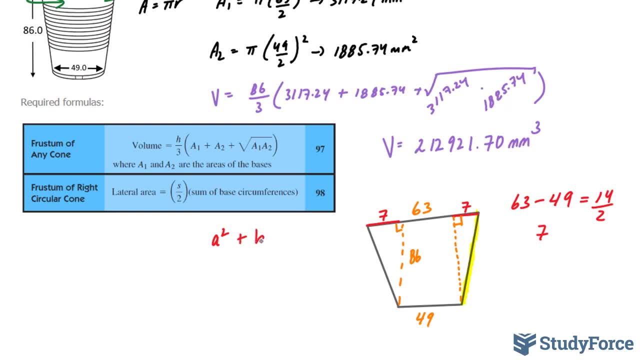 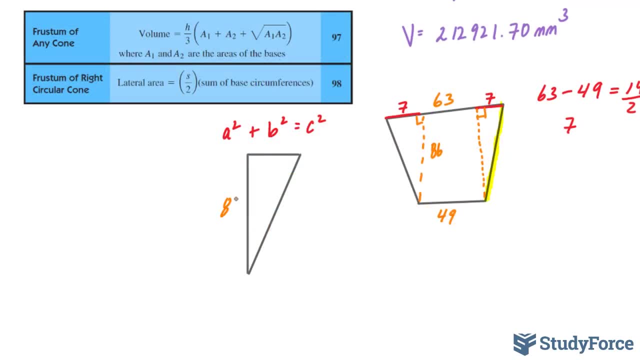 the Pythagorean theorem looks like this: a squared plus B squared is equal to C squared, and I'll draw for you just this part right here. here we'll have 86, here we'll have 7, and this given that it is the hypotenuse. 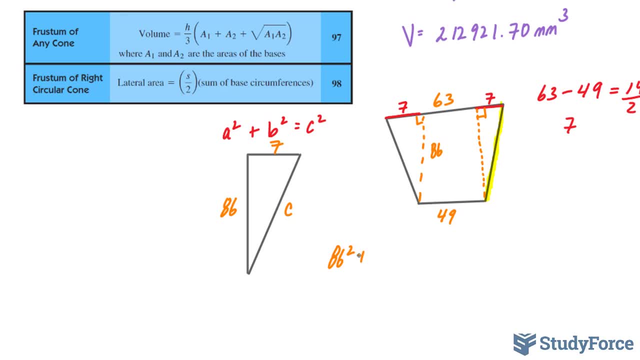 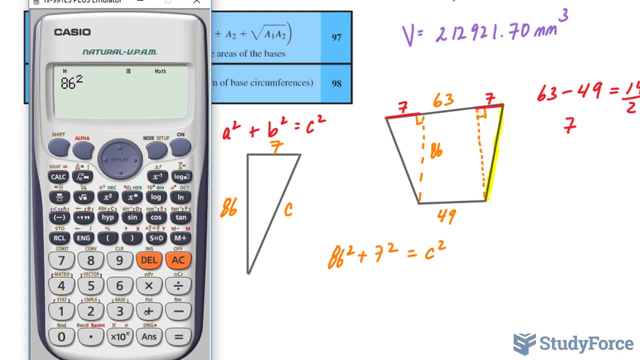 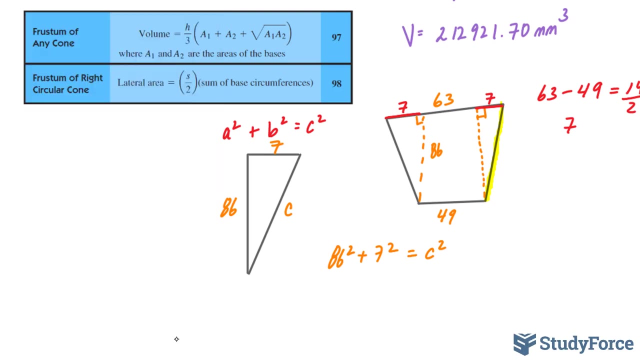 we'll call it C 86 squared plus 7 squared is equal to C squared. we'll sum these up: 86 to the power of 2 plus 7 to the power of 2 square root, that we have our hypotenuse of 86.28, 86.28 millimeters. now we can finally use this. 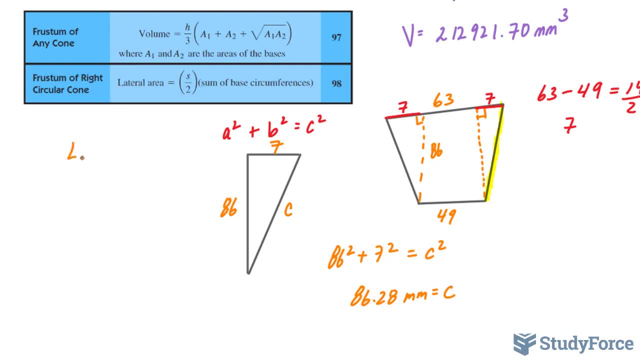 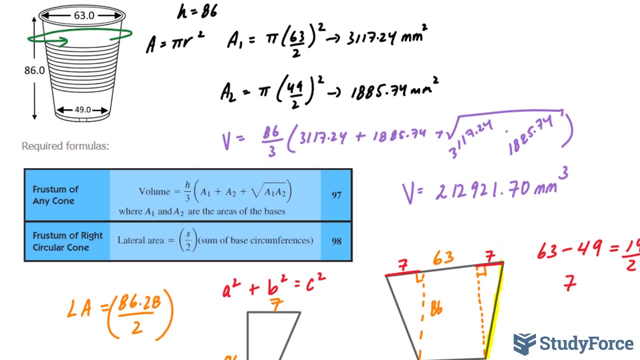 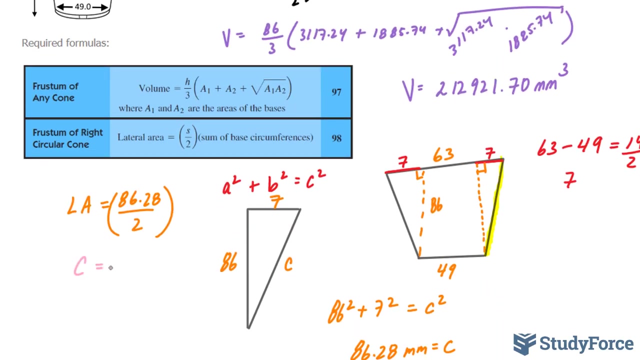 formula for the lateral area, where we have LA, which represents lateral area 86.28 divided by 2 times the sum of the base circumferences. this means going back to our diagram. here we need to find the circumference of this and the circumference of this, and the formula for circumference C is equal to PI D. now